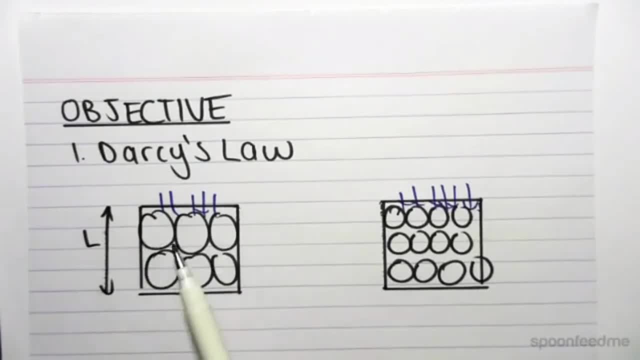 as well as the actual soil particles themselves. It's going to be a lot quicker for soil to flow through bigger particles right, Whereas when you have a more condensed soil sample with smaller particles is going to take longer for the water to find its way. 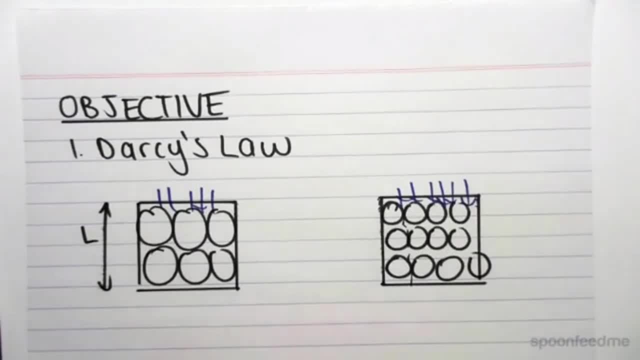 through. So we can say that the velocity is equal to k, which is a proportionality concept which we're going to define in a second, which takes into consideration the different soil samples we have, based on their particle sizes, if you want to think about it like that, as well as 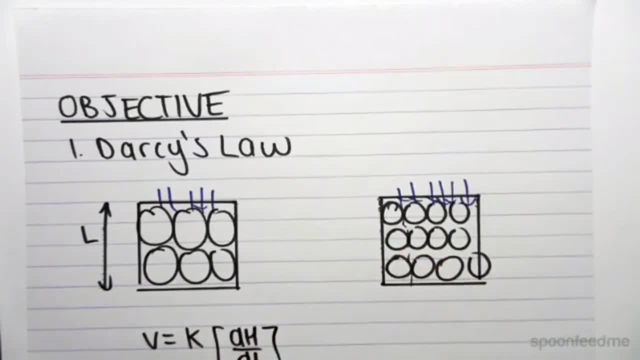 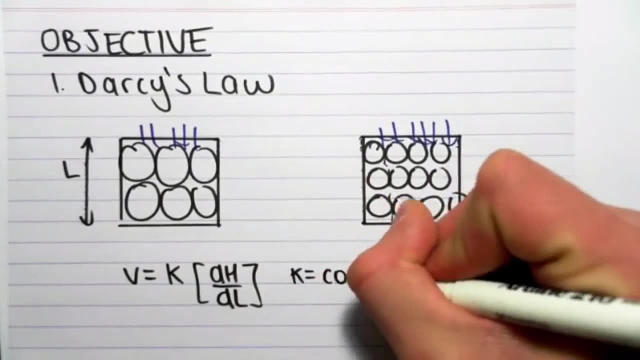 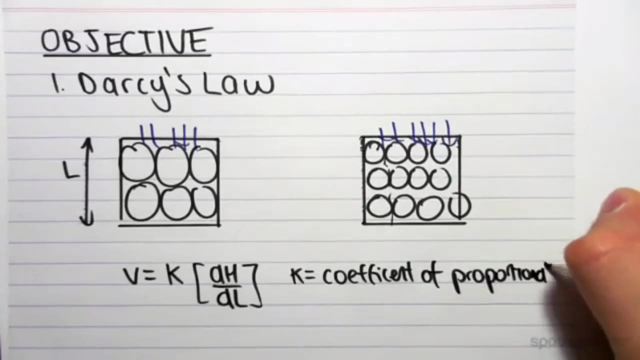 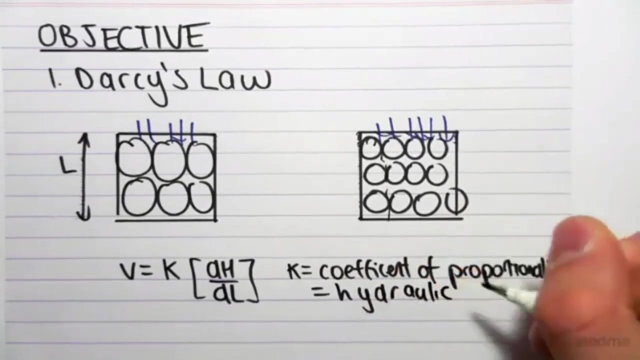 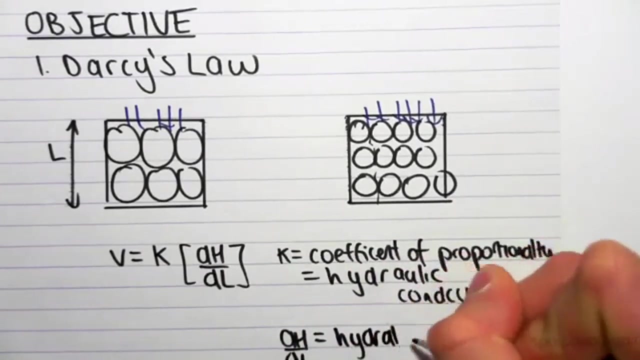 the change in head divided by the change in length. So k is equal to the coefficient of proportionality, or it's called the hydraulic conductivity. That's what k is. So k is dependent on the actual soil sample And dh hello is known as the hydraulic gradient. 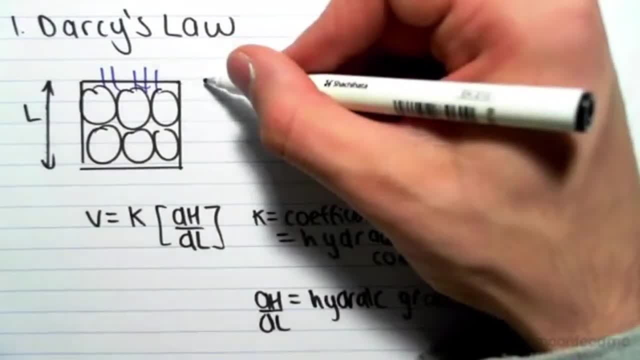 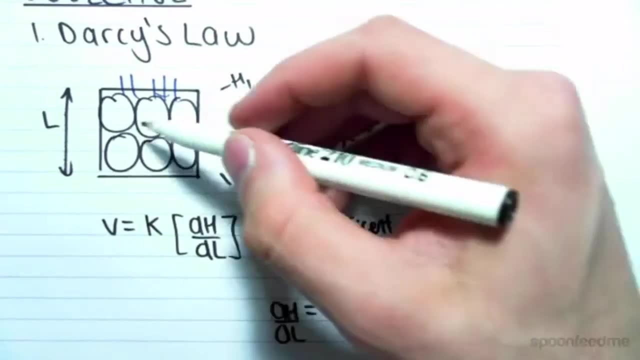 k. So it's the change in head. So say the head, say we have a head value here and head value here, and it is that change of head which causes flow divided by the change in length. So from that point to that point the change in length would be: 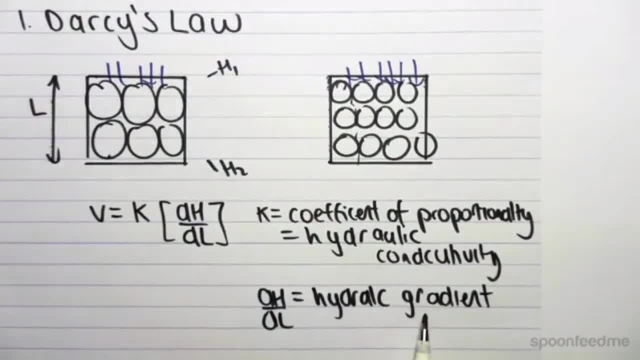 L. Just a note: this hydraulic gradient is actually unitless because heads. the unit of head is metres and the unit of length is metres. dates murderer could have had a moose, and you haveác length is also meters, so that's just going to cancel out, which means that the velocity 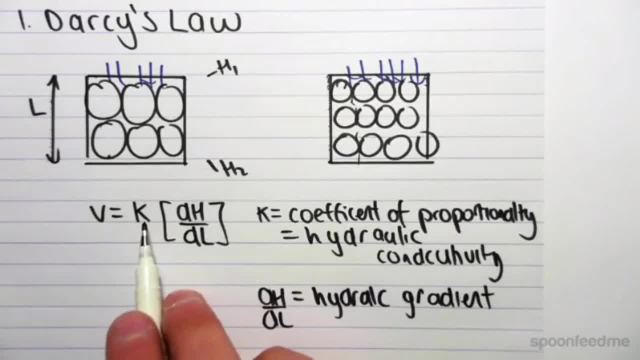 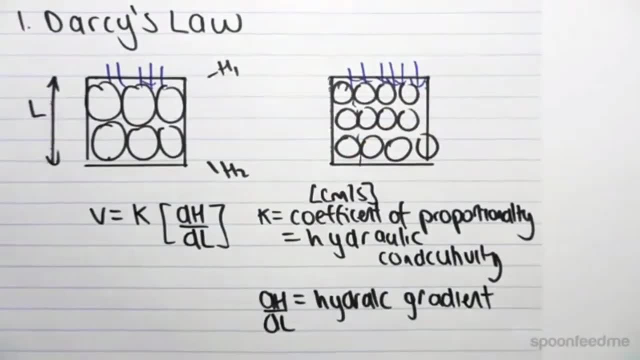 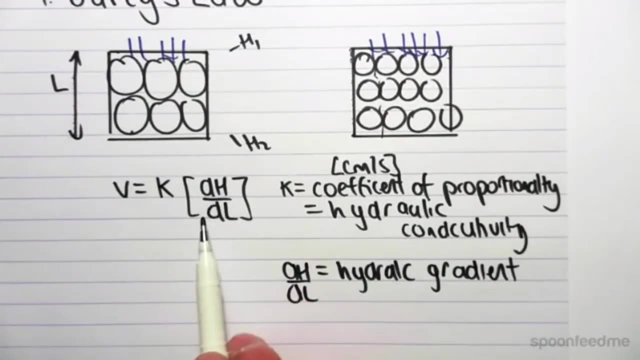 which is in, say, centimeters per second. k obviously has to be that unit as well, So k is in centimeters per second. okay, So we now know that the velocity through a soil sample is dependent on the hydraulic gradient, which is dh, on dl, as well as this coefficient. 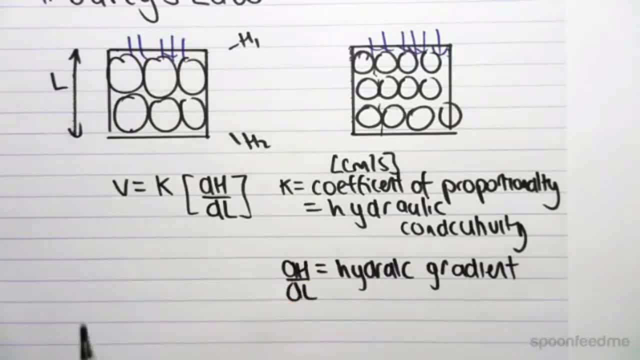 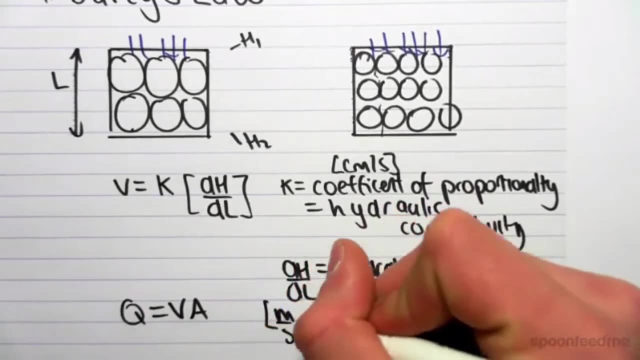 of proportionality which considers the actual soil sample. okay, Just as a side note, we know that q equals va, So q, the flow rate, is the same as the velocity times the area. This, unit-wise, makes sense. Velocity is meters per second Area, is meters squared which.